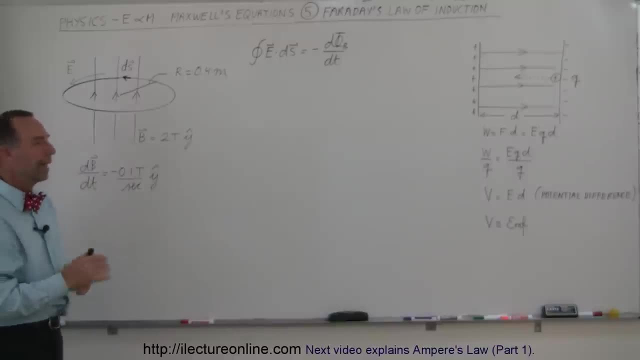 Now, if the B-field is continuous and the B-field is not changing, then nothing will happen in the loop. There simply will be a B-field and nothing special will happen in the loop. There's no current flowing through the loop, There's no potential difference or EMF across the loop. 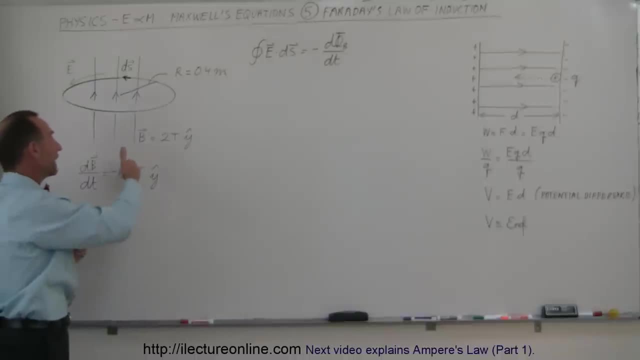 But once the field begins to change for some reason, if the field increases or decreases in such a way that the magnetic flux through the loop changes, then something begins to happen, And that's the concept of Faraday's Law. Faraday's Law said that if the magnetic field through the loop, or in other words, 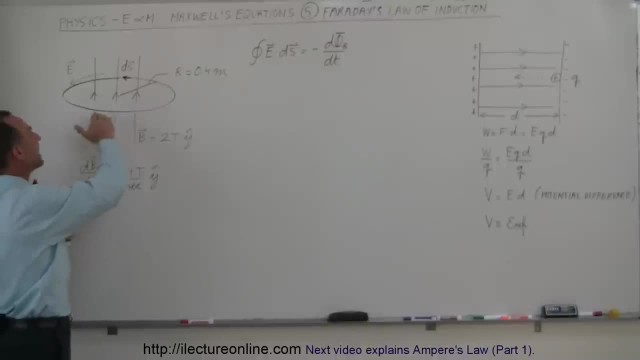 the magnetic flux through the loop changes, that will cause an EMF to be induced. And then Lenz's Law then says: well, that induced EMF will then cause a current to exist in the loop, which will then set up a magnetic field trying to pose the change of the field. 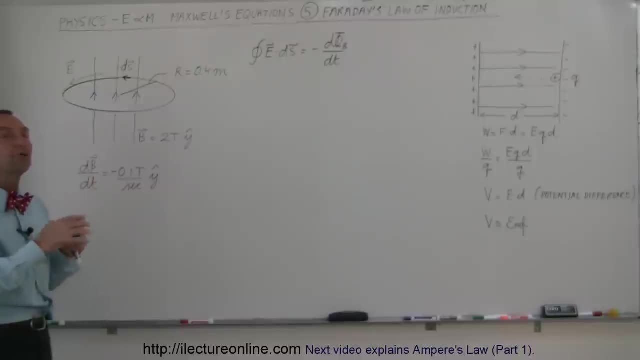 that was there in the first place, trying to pose the whole operation, trying to oppose what the field was doing in the first place, changing all right. so let's first go to an old example of how we can calculate the potential difference across, let's say, two capacitor plates where the existing 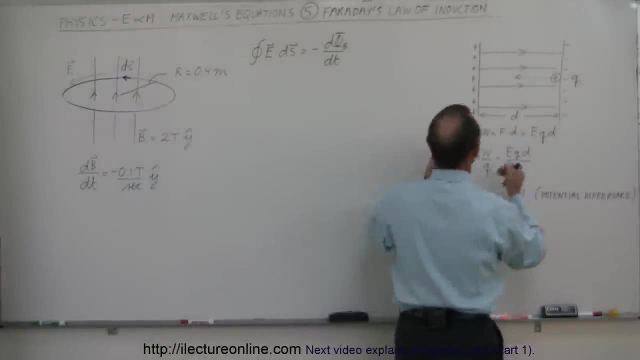 electric field in between. so here i try to draw that as an example. let's say we have two capacitor plates. let's say that there's an electric field that exists from, that emanates from left to right, and that would be what you'd expect, because there's positive charge on this side, negative. 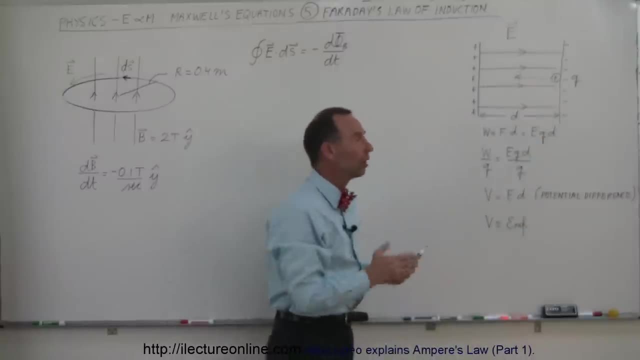 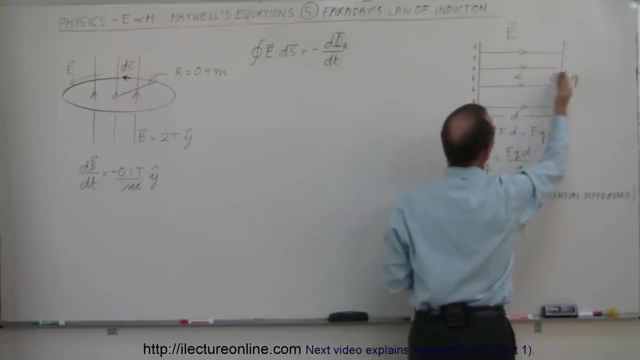 charge on this side, so we expect to have a uniform electric field between the two capacitor plates. if we now take a test charge, a small positive charge called q, and we push it all the way across from the negative side of from the negative plate to the positive plate, we would have to do a. 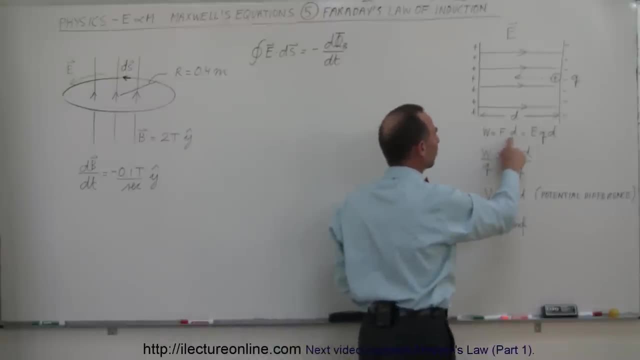 certain amount of work. that work will equal to the force times the distance, and the force exceeds the negative side of the negative plate. so we would have to do a certain amount of work. by the small test charge inside electric field, e would equal e times q. that's by definition, and 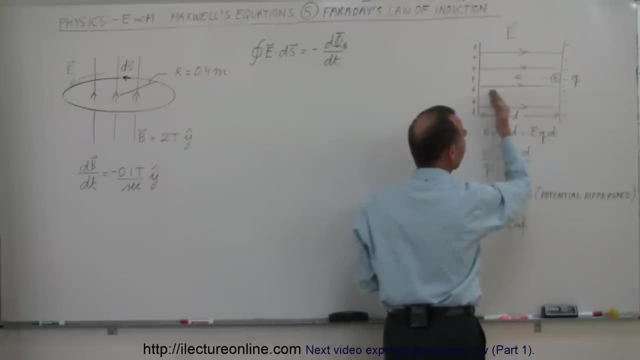 of course we take the force e times q, multiplied times the distance traveled, d. that will then be the work done to get that small charge from this side to the other side right there. if we now just divide the work done by the test charge, q, that's the same as saying eqd divided by q and by definition, 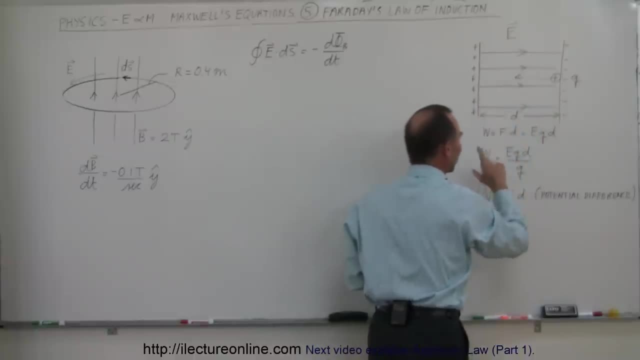 the work done to move the charge from there to there, divided by q, equals the potential difference between the two plates, and i indicate that by v, which is the voltage between the two plates, which is therefore equal to e times d, since the q's cancel out, and that is then known as the potential. 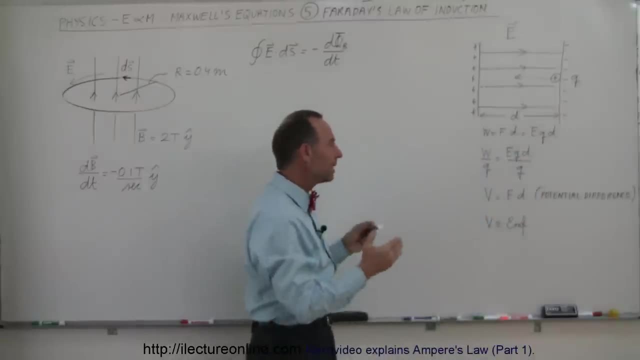 difference between the plates. it can also be assumed to be the emf between the plates, the electromotive force, and the reason why they called voltage or potential difference electromotive force, because it appeared as if, whenever there existed a potential difference between two locations, there was this apparent force trying to drive, charge it from one side. 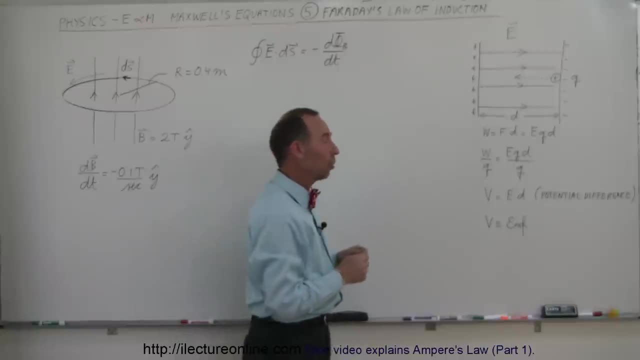 to the other, from one potential to the other, and so if it was a higher potential here, low potential there, a positive charge would be pushed in the direction from higher to lower potential. if there was a higher potential here, low potential there, a negative charge would be pushed from the. 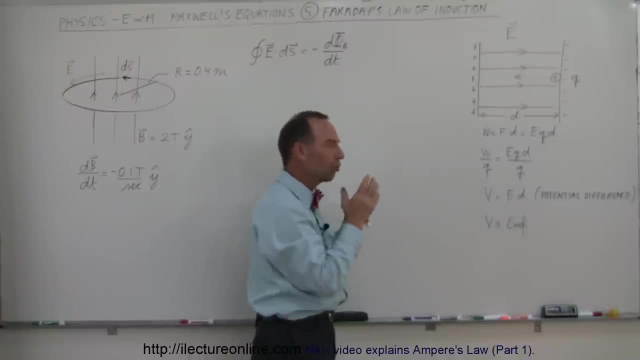 lower potential to the higher potential. so that was understood to be the potential difference and that was understood as also to be the emf, the electromotive force seeming to drive charges from high to low, from low to high, depending upon whether or not they're positive or negative. 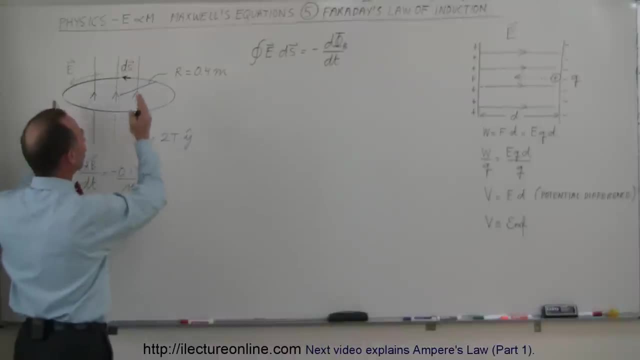 so, keeping that in mind, now let's go back to what we call faraday's law of induction. now the magnetic field changes as the magnetic field changes. let's say, for example, that the change in magnetic field is equal to of minus 0.1 tesla per second. that will then cause the magnetic 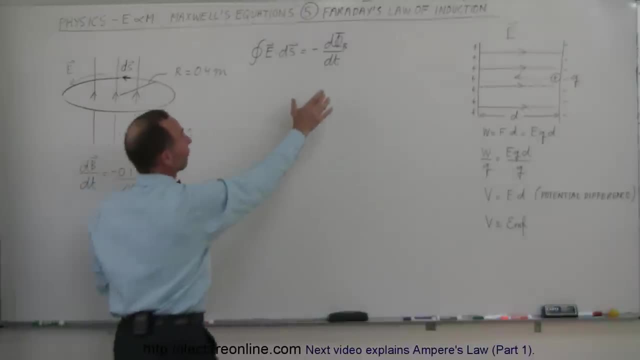 flux to the loop to change, which will therefore, based on faraday's law, cause an enf to be induced and the surface- not the surface integral, but the line integral of e dot ds- is then equal to minus the change in the magnetic flux over time. now, if you don't remember what the 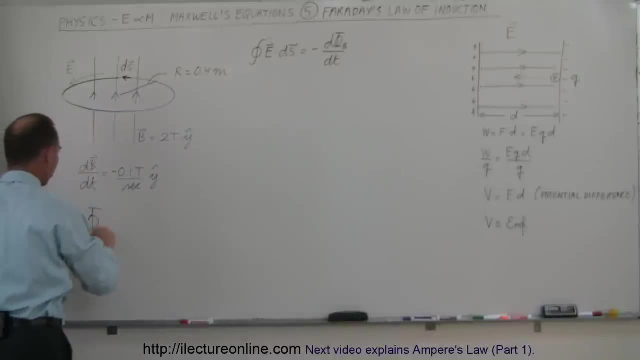 magnetic flux is the magnetic flux in this case would be equal to the magnetic field strength, b times the area of the loop a. so in this case that would be equal to b times the area of the pi times the radius squared. and since we have given you these specific amounts here, you can say in: 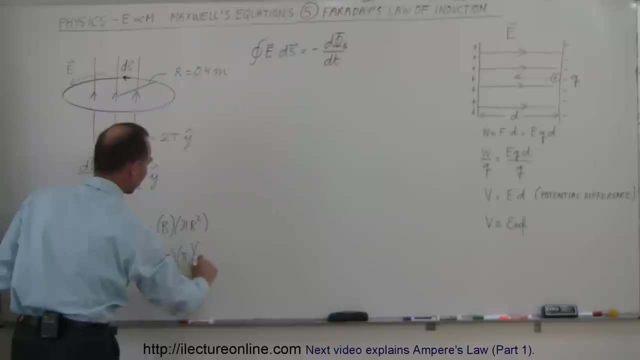 this case, that would be two teslas times pi times 0.4 meters squared, and that would be the magnetic flux through the loop. and, of course, as the magnetic field strength is decreasing by 0.1 teslas per second, we can expect the, the flux, the magnetic. 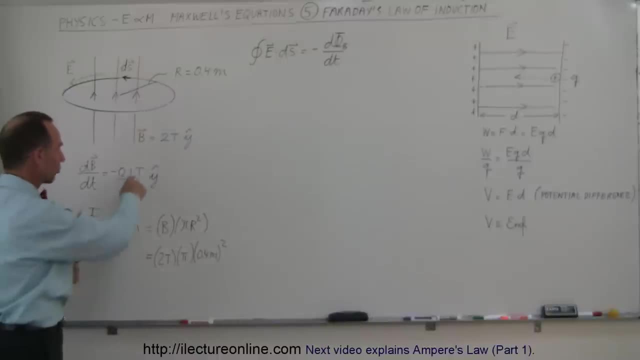 flux of the loop to decrease in the same ratio. this looks like it's about 120th or about five percent per second. so the magnetic field will lose its strength five percent every second. so that would happen over a period of about 20 seconds. the same would happen to magnetic flux. it would. 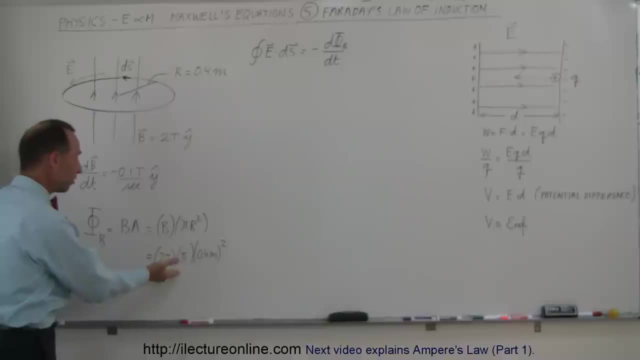 decrease at a rate of five percent per second and it would go from this amount to zero in 20 seconds, just like the magnetic field. while that is happening during those 20 seconds, while the b field is changing, while the magnetic flux is decreasing, that would cause an electric field to exist. 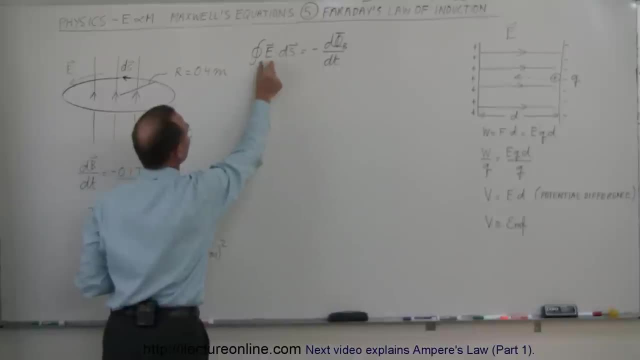 along the loop. and if we take the strength of the electric field and multiply it times the circumference- because that's where the line integral is, we can assume, since the distance, since the the loop is perfectly symmetric all the way around, it's going to decrease at a rate of five percent per second. and if we take the strength of the electric field, 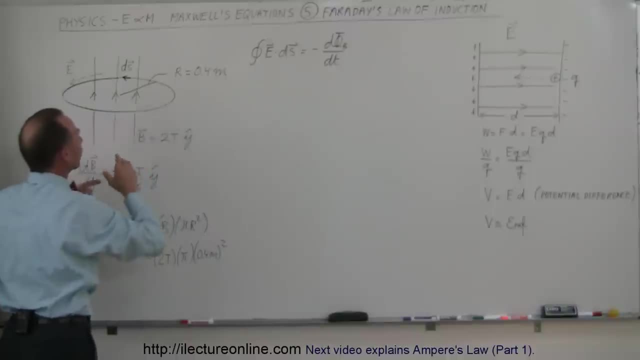 to circle a loop. the b field is- is uniform throughout the loop, we can expect the strength of the electric field to be the same everywhere along the loop, of course the- the direction of the electric field of course will change- will be parallel to the, to the current loop, all the way. 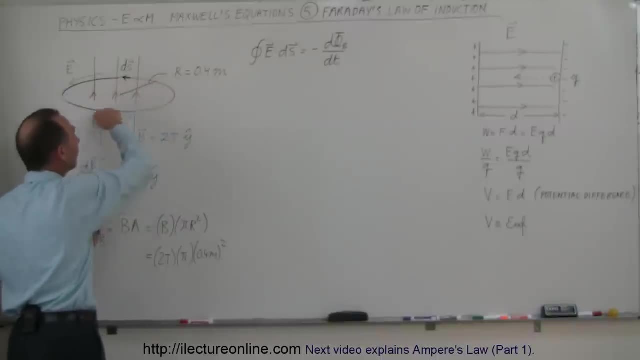 around. and if we then multiply that, times the entire circumference e times the entire circumference two pi r would equal the line integral of e dot ds. so what we can say then is we can say that the strength of the e field along the electric field is going to decrease, and if we then multiply that, 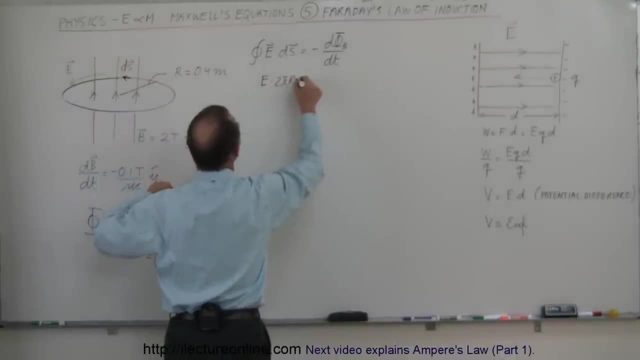 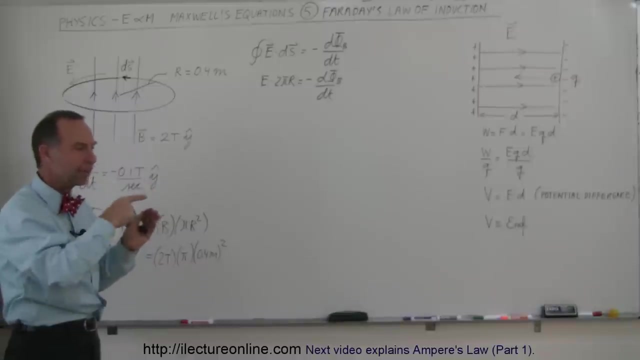 along the loop times the circumference, 2 pi r. that is equal to minus the change in the magnetic flux over time. now, what is e dot 2 pi r? it's the strength of the electric field times the distance of that path. that sounds an awful lot like what we just did over here. 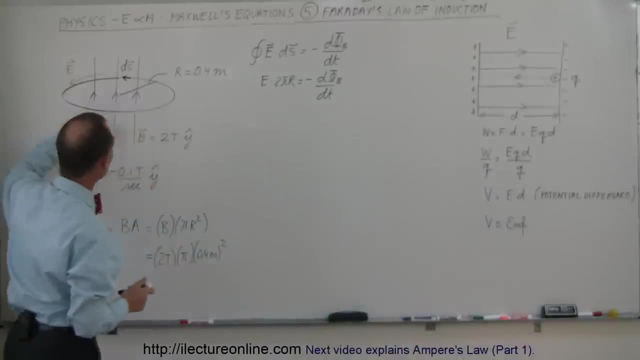 because here the electric field is uniform and over here, along this current loop, we can say the electric field is uniform as well. it's the same, at least in magnitude, of course. of course it changes constantly in direction, but that's okay, because anywhere we go along the loop, 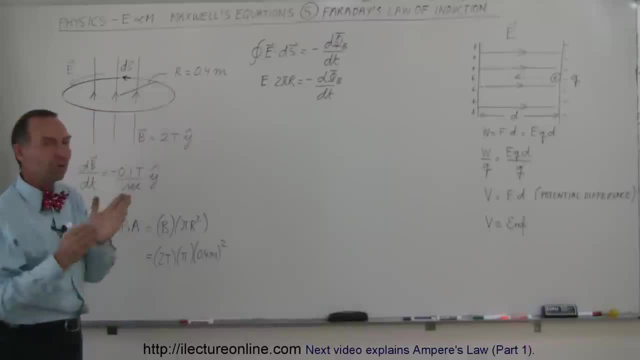 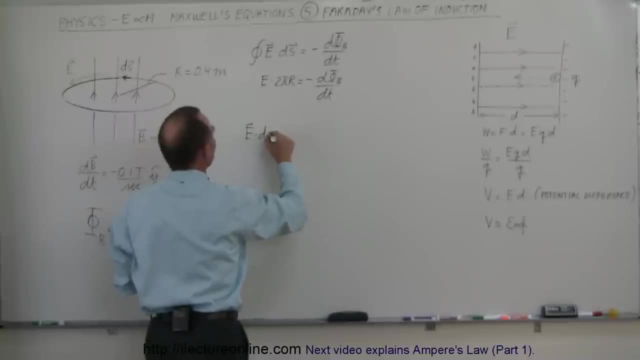 the e will always point in the same direction as the ds, and so therefore, the angle between them is zero, and so e dot ds, if we want to write it like this, e dot ds is equal to the magnitude of v times the magnitude of the s times the cosine of the angle between them. but you can see that. 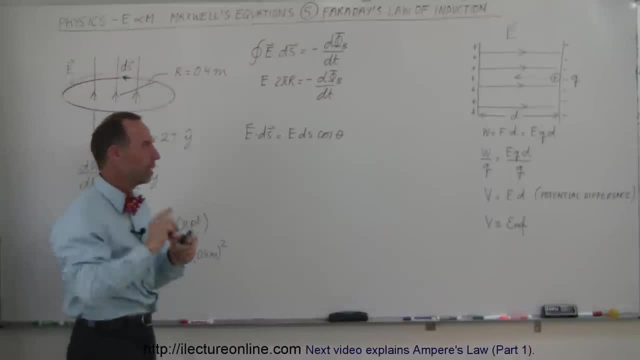 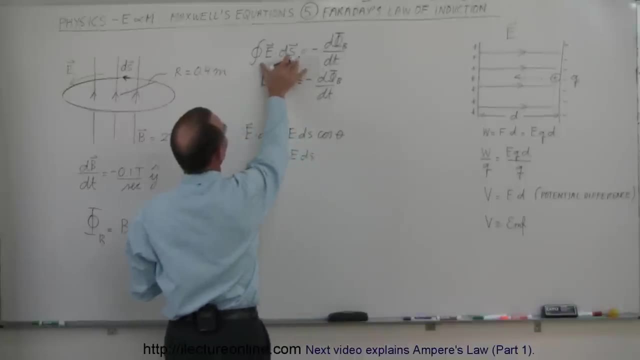 the angle between the two is always zero all the way around, then the cosine of zero is one. so in this case we can say that's equal to e times the ds, and then of course that would be a small, uh infinitesimal small section of this whole. 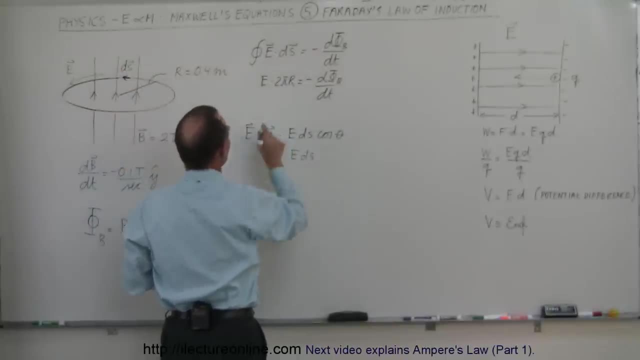 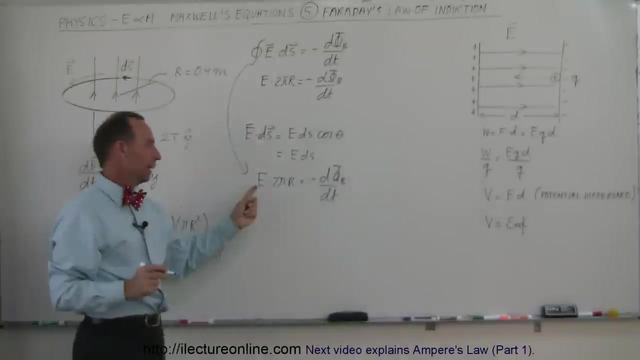 circumference. if we then integrate all the way around, we can then say that this integrated is equal to e times the complete circumference, 2 pi r, which is what we write over there, which is equal to minus the d dt of the flux, magnetic flux. now, if the strength of the field 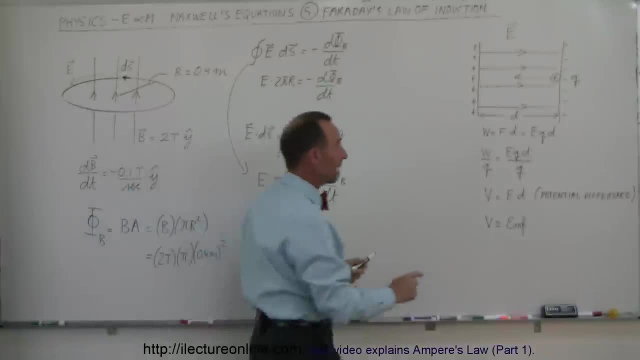 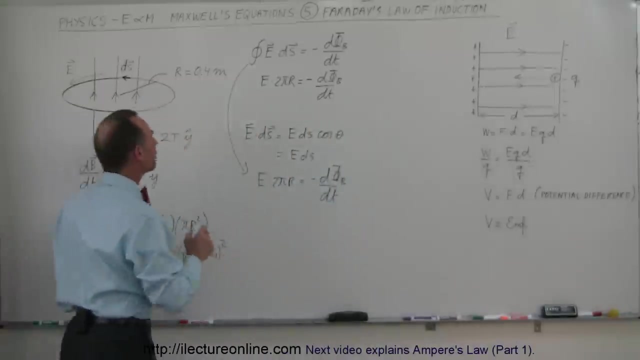 doesn't change and you multiply it times 2 pi r. that's the exact same thing as saying the strength times the distance traveled, which means that this has to be equal to the potential difference, which means that, because of the change in the magnetic flux, it is as if there is a potential difference across this loop. it is as if we added a battery. 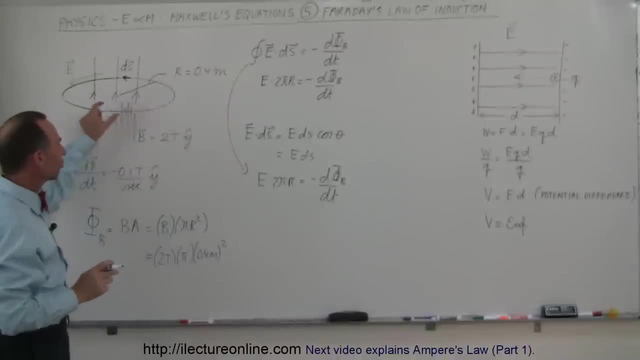 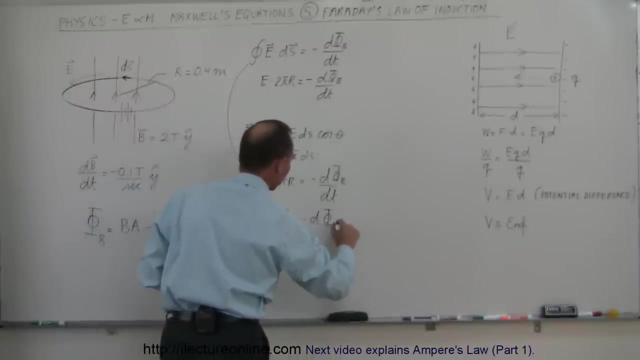 on this loop and the strength of the battery. the potential difference of that battery would be equal to the emf induced, which in this case is equal to e dot 2 pi r. that will then be the emf minus the change in the magnetic flux over time, and so the strength of that ems the amount. 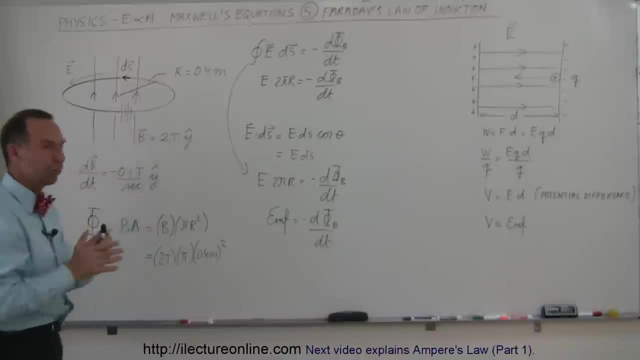 of that voltage, the amount of that potential difference. there is, of course, no real battery there, but it acts as if there's a real battery there, causing the current to flow around. now, if the electric field is going in this direction, that means us higher pos, that's higher potential here. 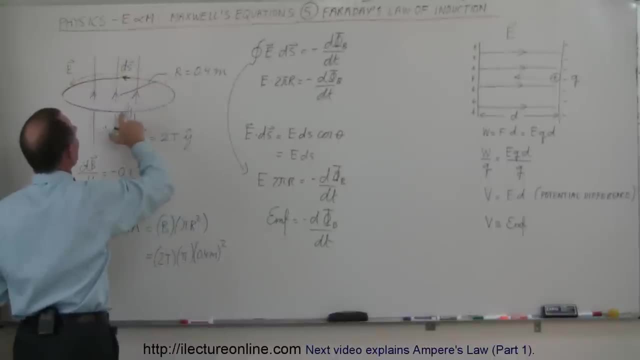 lower potential there. so in essence, i guess i should have drawn the battery this way: where the positive side of the battery is here, the negative side of the battery is there, so that we have the direction of the change in potential in that direction. but now, can we figure out how big that is? yes, we can. we just need to know what. 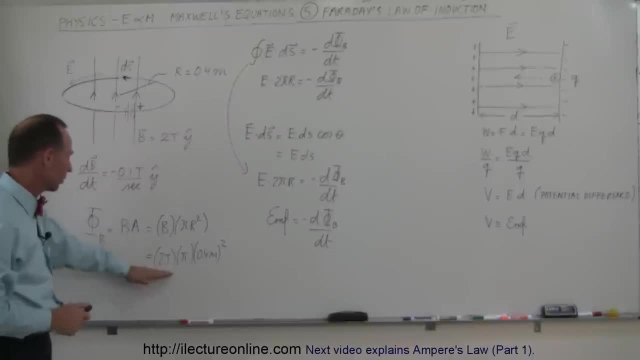 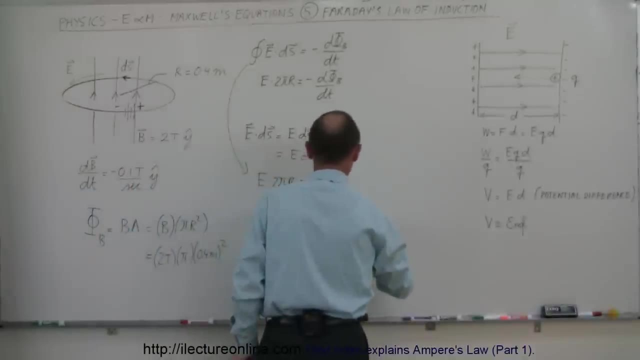 this change in the the flux is and, of course, since the flux is equal to this and it changes by five percent of this every second, we can therefore say that this is equal to 0.05, which is five percent of the total amount that it started with. so five percent of two, that's two teslas times pi. 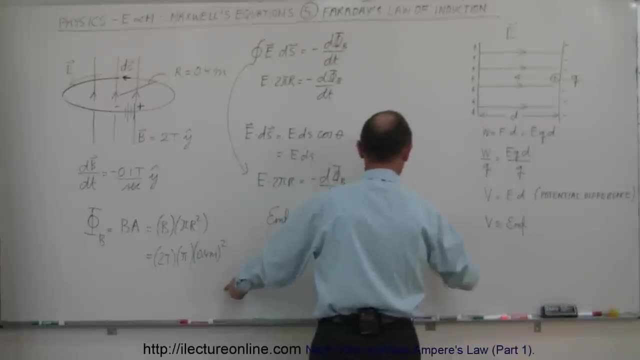 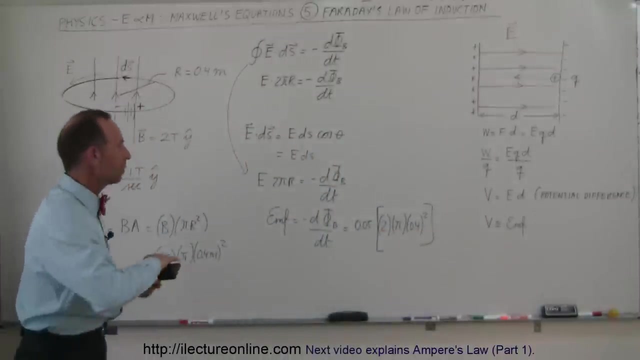 times 0.4 squared, and of course that would be meter squared. so, teslas, meter squared and times five percent, and let's see what that would be equal to now, where? what about the negative? well, we can still put the negative there. it just simply means that the it's simply a. 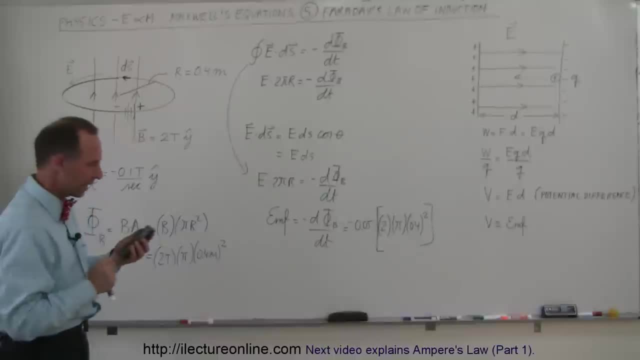 reactionary thing to the change in the magnetic flux. that's why the negative is there. It's kind of like the same thing with the spring constant. The force is equal to minus kx. That's because it's a reactionary force. EMF induces a reactionary event to the 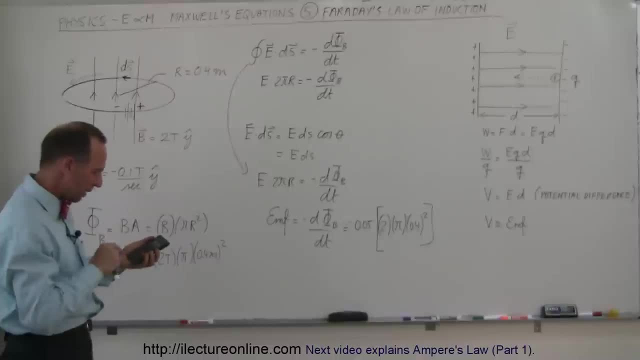 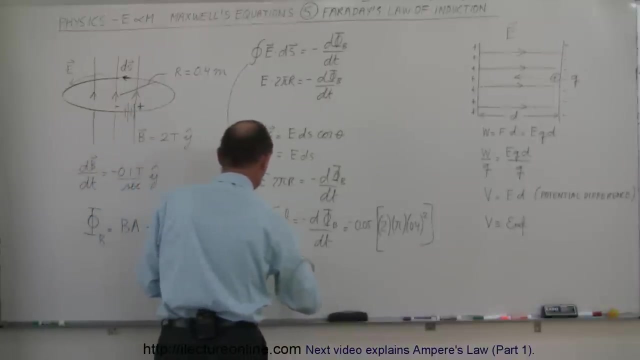 change in the magnetic flux. That's why the negative is there. All right. so 0.05 times 2 times pi times 0.4, squared equals, and it looks like that would therefore induce an EMF of voltage equal to 0.05 volts. So by allowing the magnetic field to change at a rate of 5 percent per second, 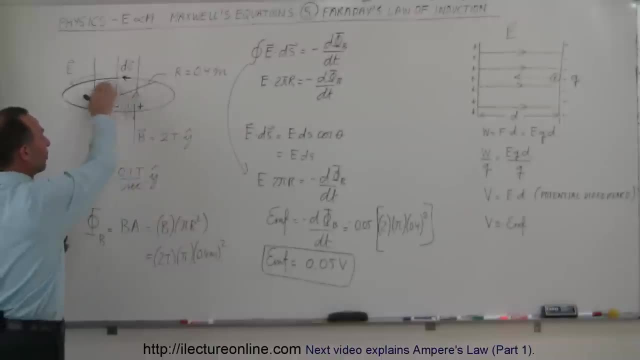 over a period of 20 seconds, from 2 tesla down to 0, changing the magnetic flux to the loop, you will for those 20 seconds, induce an EMF of 0.05 volts, which will then cause a current to. 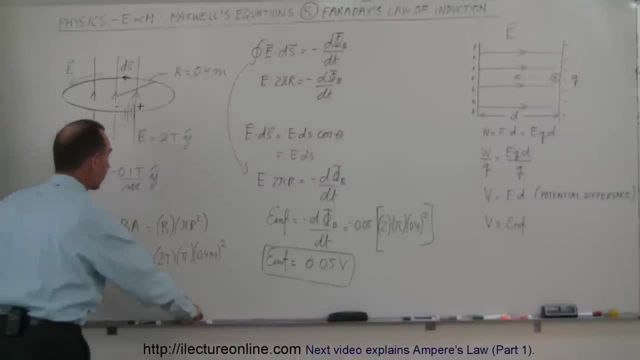 flow through the loop. And now let's take a look at that real quick. So then you would have a current flowing through the loop like this, Which will then set up its own magnetic field which will oppose the change. Now, that's Lenz's. 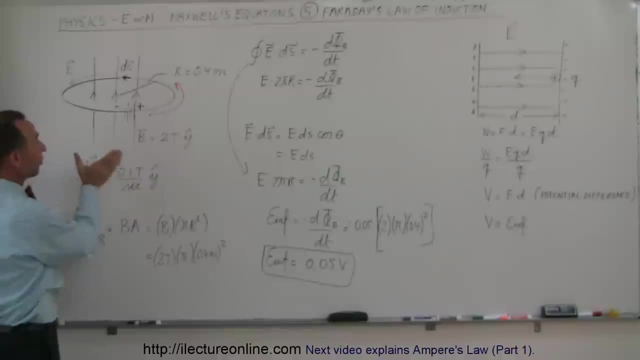 law. And what you can then do is look at this: If there's a current going through the loop like this, use your right-hand rule. if the current goes around like this, your thumb will then point in the direction of the B field produced by this induced current. So now you'll have a B field. 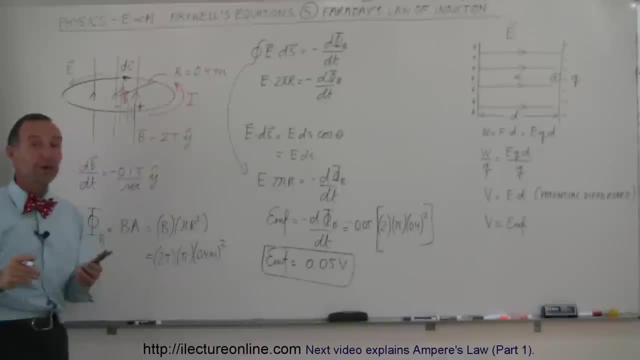 which will be in the same direction as the original field, because this current will produce a B field that will try to oppose the change. What is the change? A reduction in the strength of the field. And opposition to the reduction strength of the field is adding additional B field to try and keep it from reducing. 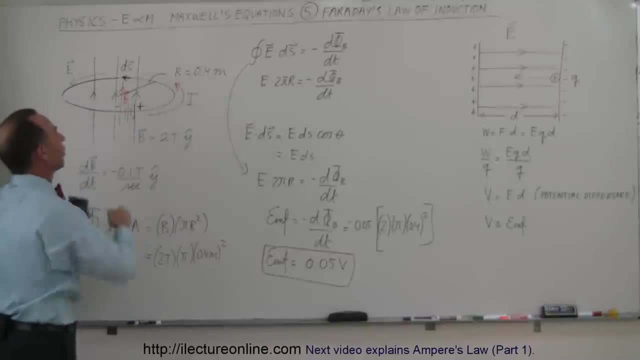 Of course, that's only a temporary thing. Eventually, the B field will always go to 0, but at least induced current, which is a product of the induced EMF, which is a product of the induced electric field around the loop, like that, will therefore exist and set up a